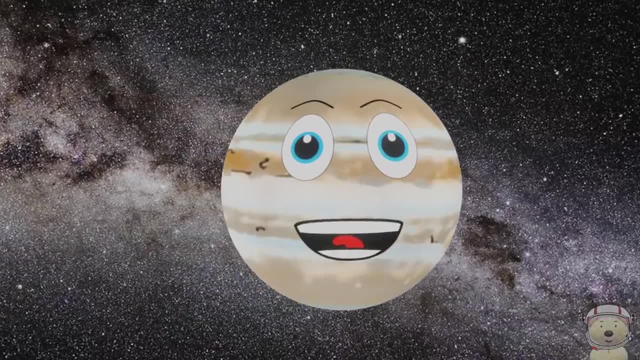 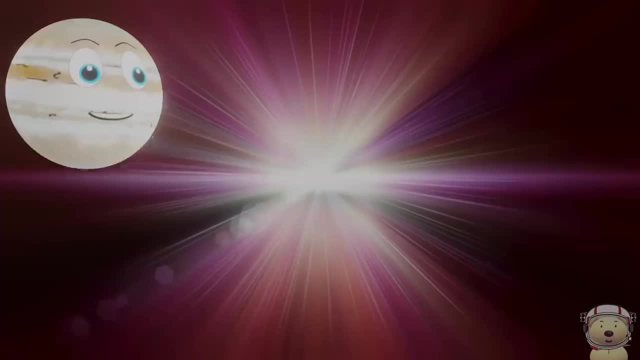 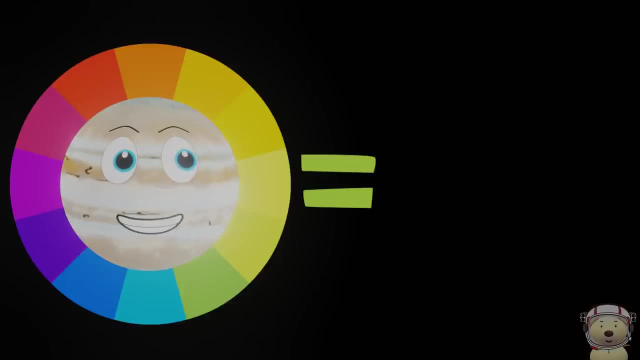 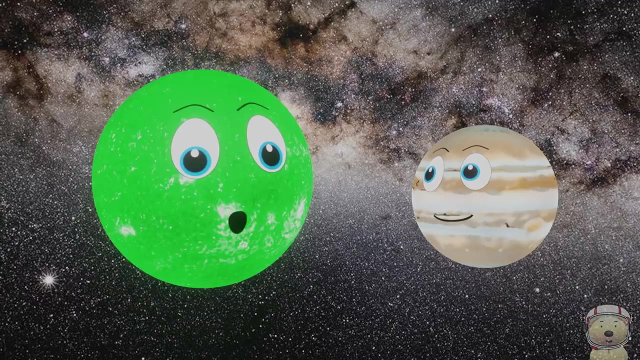 Wrong. The real colour of the sun is actually well white. What The sun sends out, all colours of the rainbow and all colours of light combined, make white light. If the sun was a certain colour, say green, The sun is Hulk, Hulk smash. 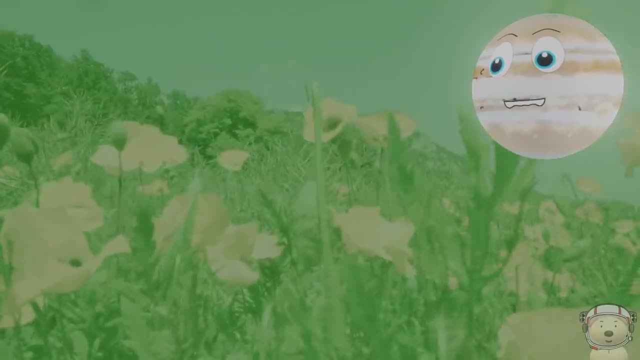 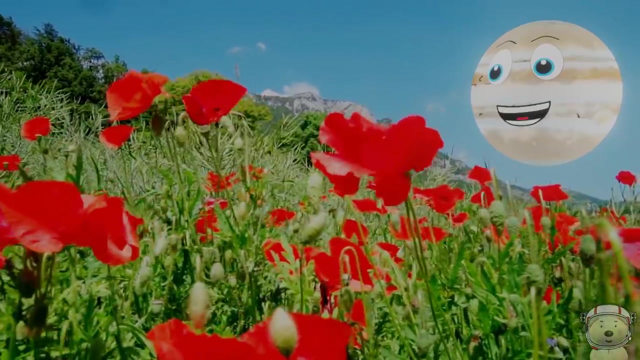 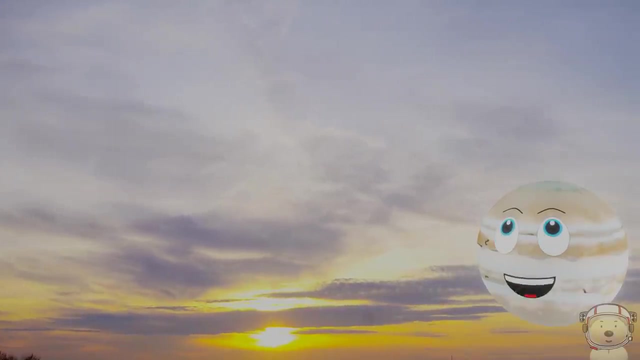 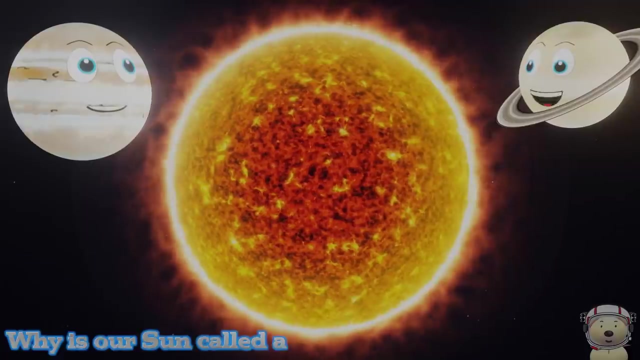 Uh sure, Then everything on Earth would look green or dark. But because it's actually white, we can see all the colours on Earth. The reason it looks yellow to us is because of the Earth's atmosphere That is far away. Why is our sun for the yellow dwarf star then? 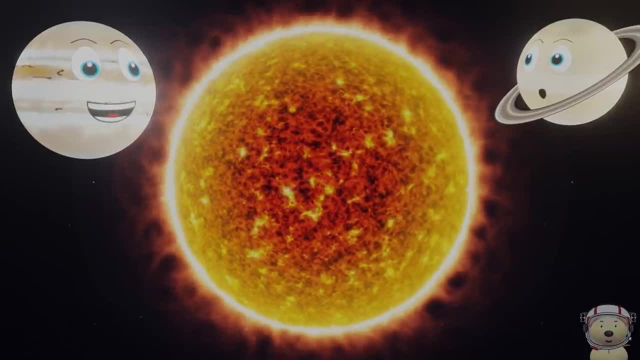 Well, not all yellow dwarf stars are yellow. Well, not all yellow dwarf stars are yellow. So are white, and our sun is one of these. So are white, and our sun is one of these. So are white, and our sun is one of these. 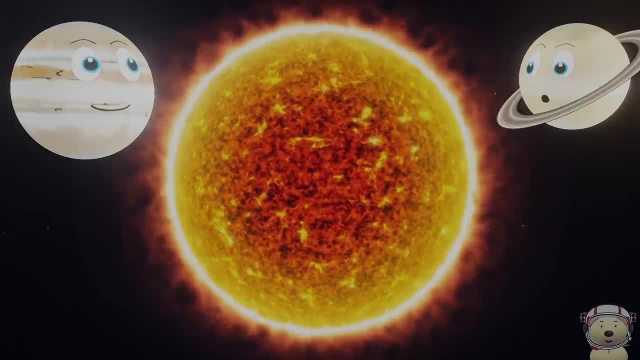 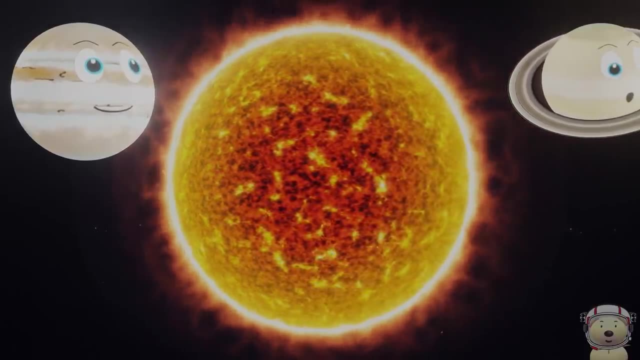 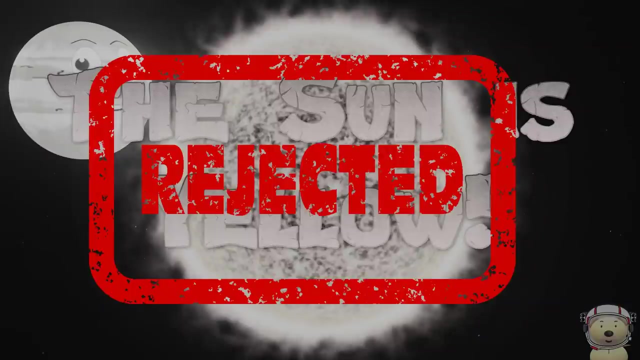 Confusing. So it's a yellow dwarf And it looks yellow to us, but it's not actually yellow, and it looks yellow to us, but it's not actually yellow. ra-r praying Fact checked. Question 3: The asteroid belt is dangerous. 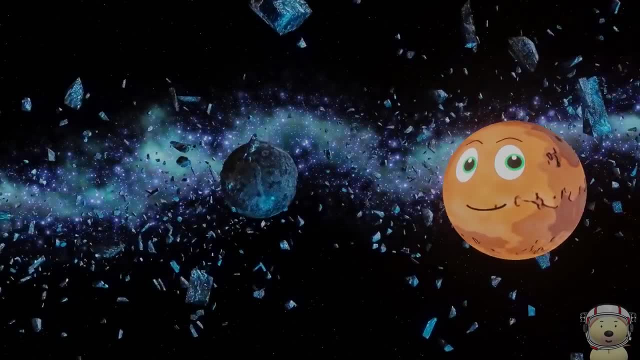 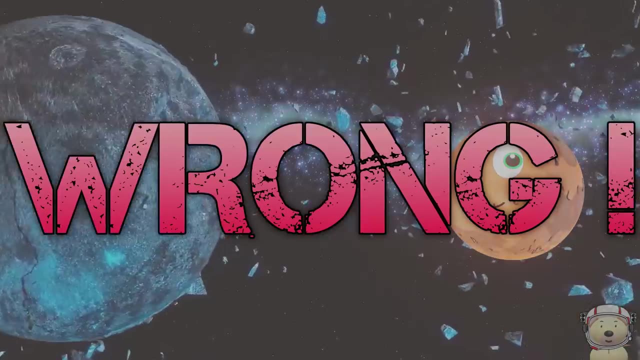 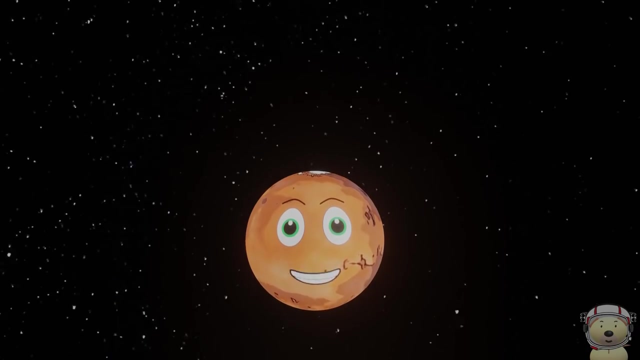 The asteroid belt is dangerous, Dangerous. Many people think the asteroid belt is very dangerous and it is crowded with asteroids- Wrong. Think of your favourite space movie and you will see spaceships dodging in and out of the way of asteroids Woo. 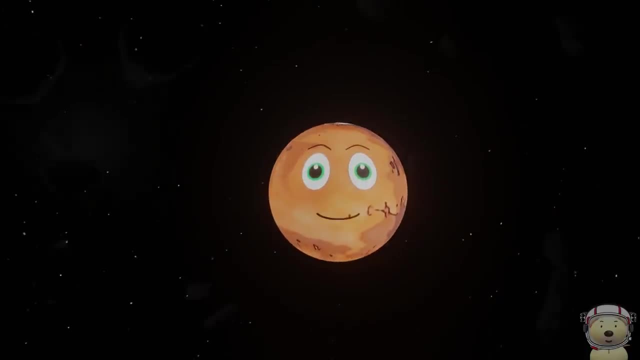 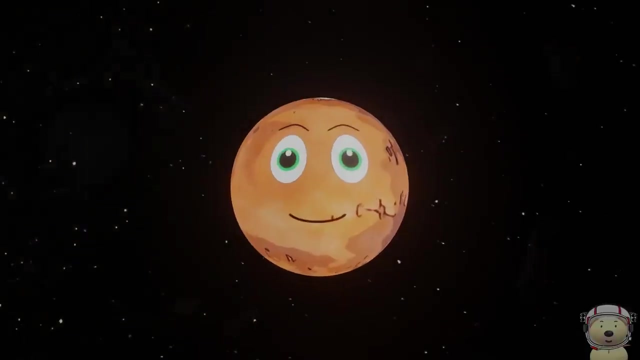 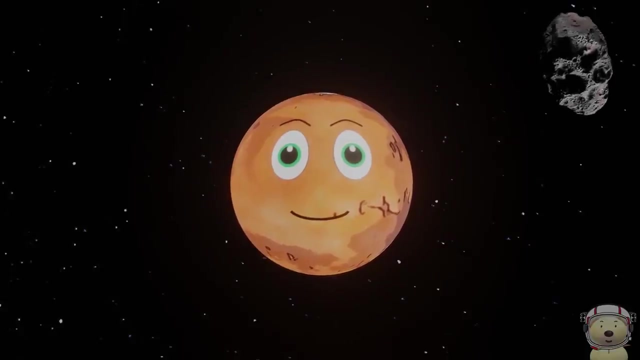 However, the asteroid belt is not like that. Several of our spacecraft, including Voyager 1 and 2, have flown right through it. The truth is, asteroids are really far apart and hitting one would be very unlikely. What Yikes. 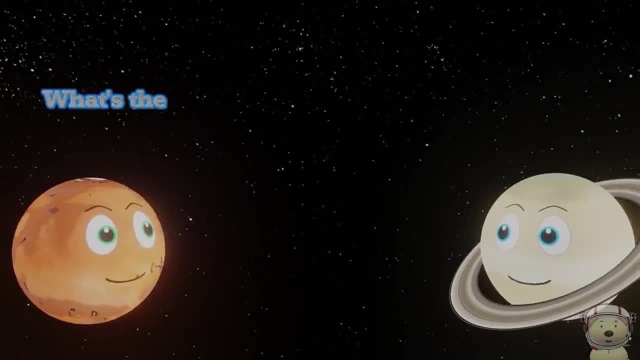 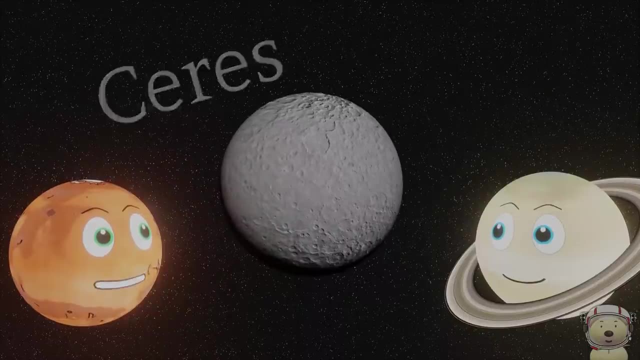 What's the largest object in the asteroid belt? The dwarf planet Ceres is the largest object in the asteroid belt. It's best to avoid an object that is too small to hit. It's best to avoid an object that is too small to hit. 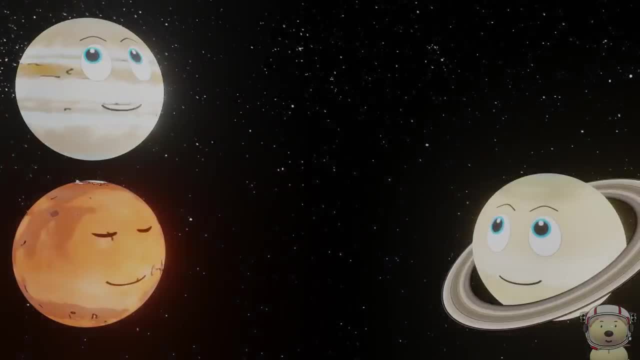 That size. Hey, Saturn, I've got a space joke for you Right. Go on then. When do astronauts eat? I don't know. At launch time, Ha ha ha. Lunch, L-Launch time, Get it, Not for me. 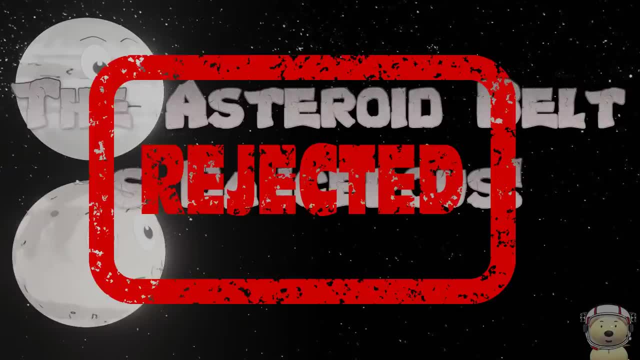 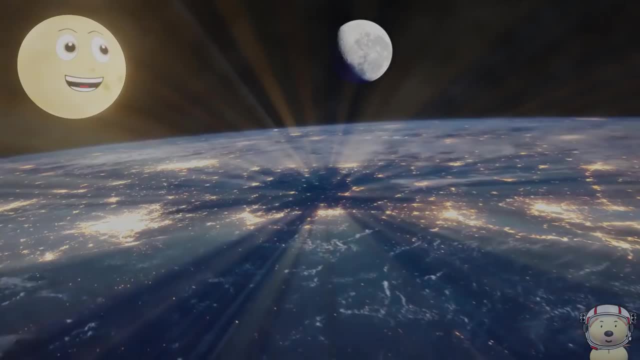 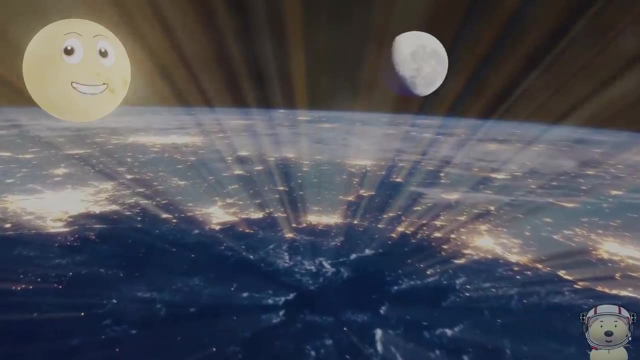 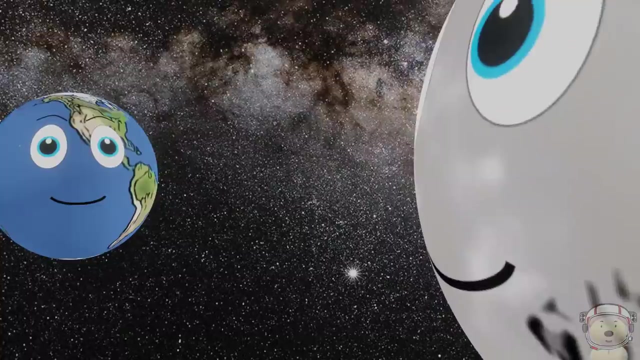 FACT CHECKED: The moon is close to the earth. Many people think the moon is very close to the earth. WRONG, Because the moon looks so big in the earth's sky, it must be close to us. Well, no, On average, the moon is about 238,855 miles away from the earth. 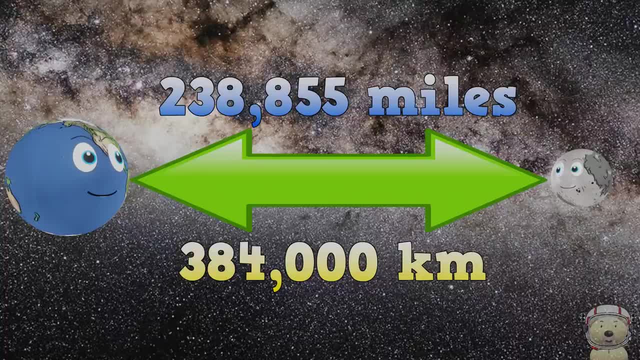 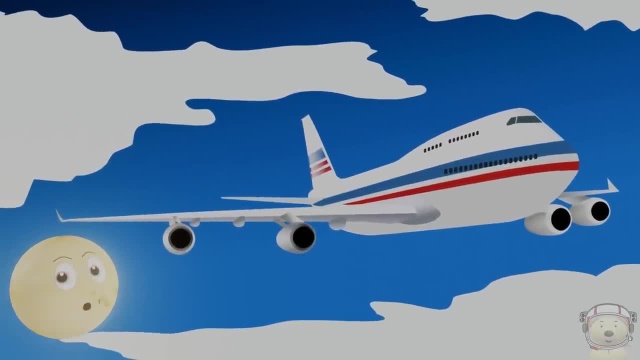 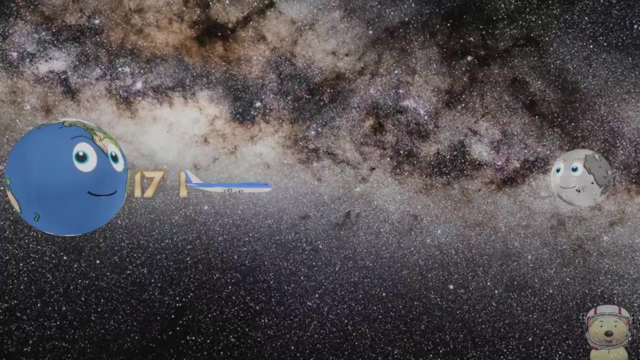 That's about 384,000 kilometres. That is far away. Look at the 747 jumbo jet that you fly to on holiday. It can fly at nearly 600 miles per hour. If you could fly to the moon on one of these aircraft, it would take you 17 days non-stop to get there. 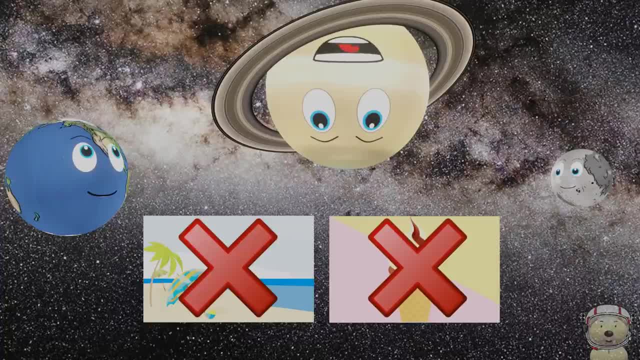 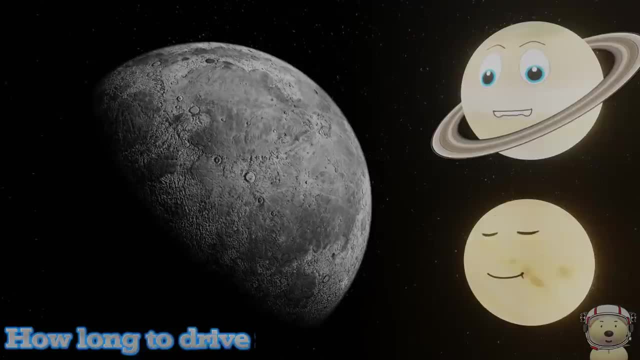 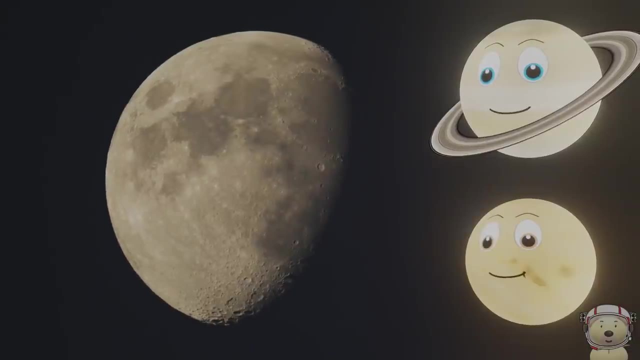 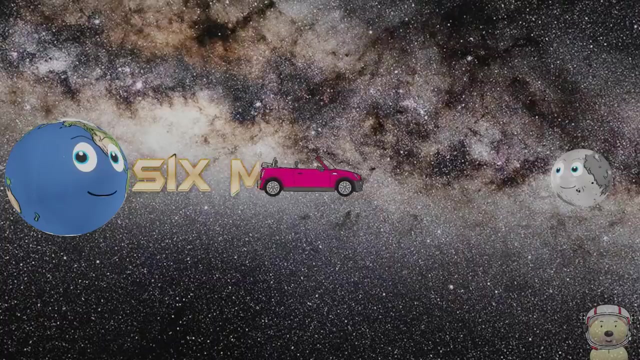 And there's no beach or ice cream there either. On a normal spacecraft, it would take you about 3 days. How long to drive in a car to the moon? Well, at 60 miles per hour, hmmm, If you could drive a car to the moon, it would take you nearly 6 months to get there. 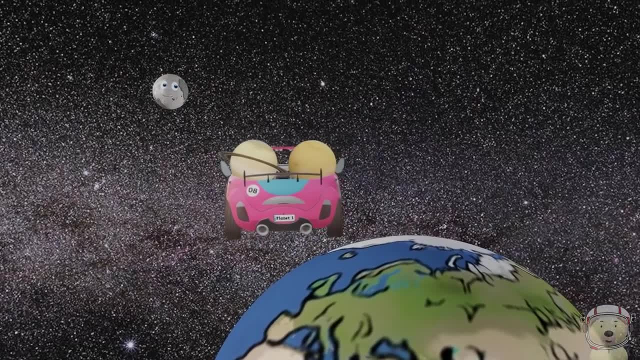 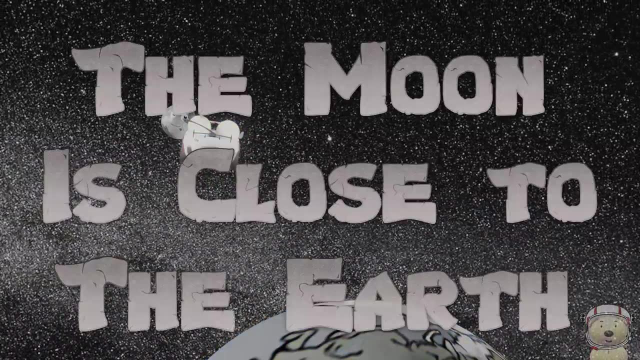 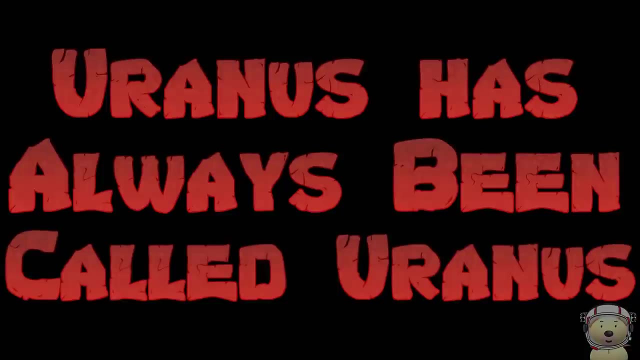 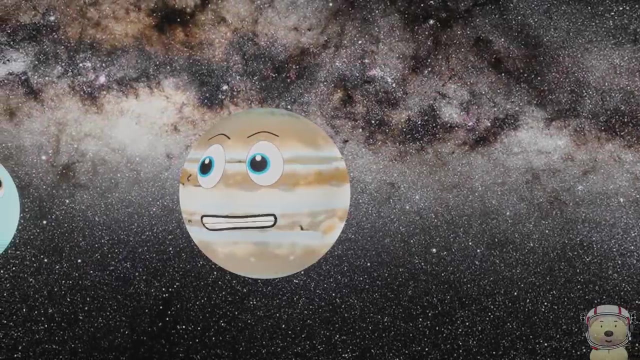 Are we there yet? No, Are we there yet? No, Are we there yet? No, FACT CHECKED: Uranus has always been called Uranus, Hi Uranus. so you have always been called Uranus, then. Well, yes. 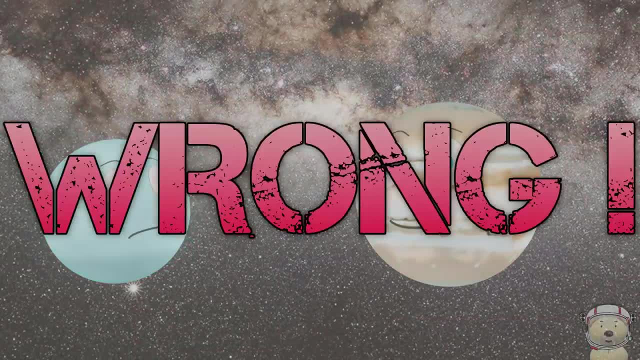 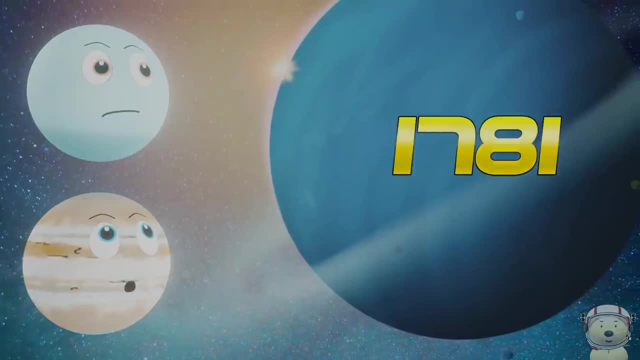 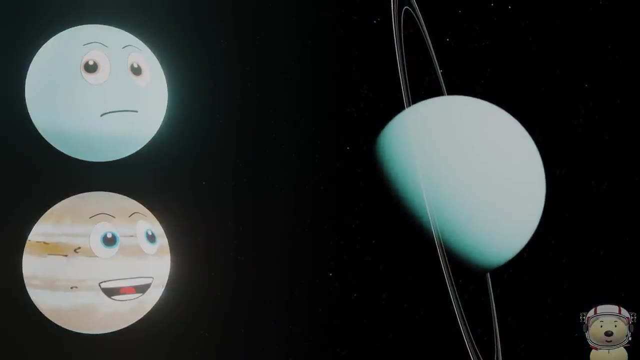 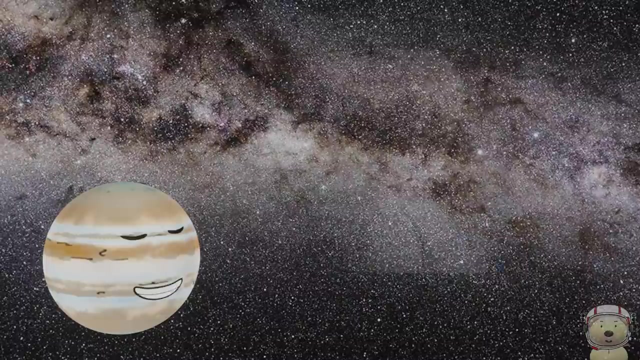 Of course I WRONG What? After you were discovered in 1781, for 70 years, you were called Georgium Sidus. Why, you ask? Well, you were named after King George III of England. So you could have been called Planet George after the King. Imagine that. 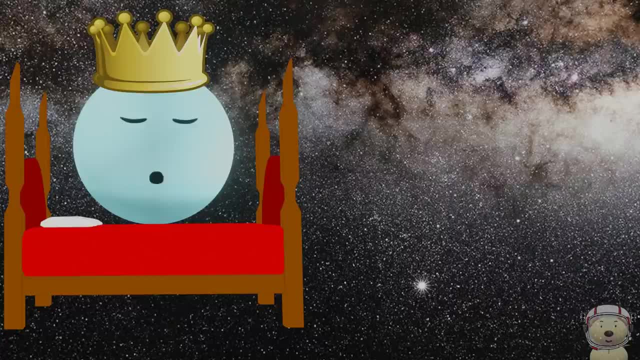 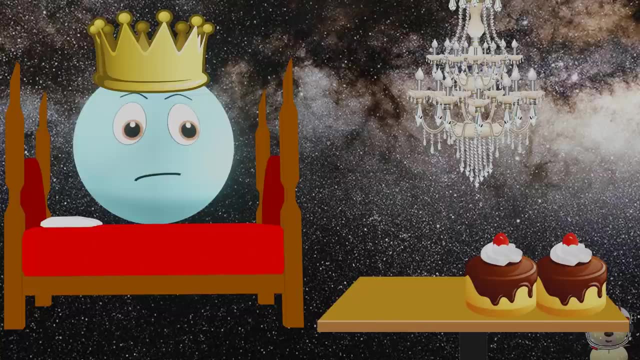 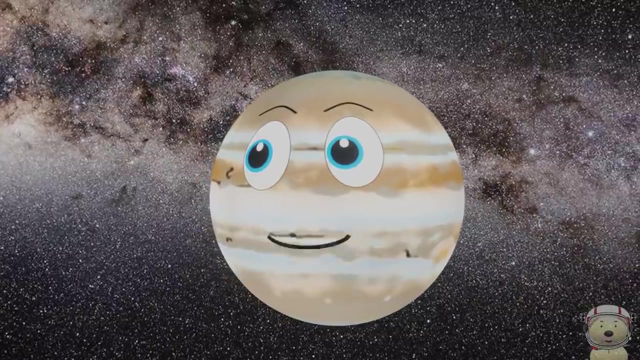 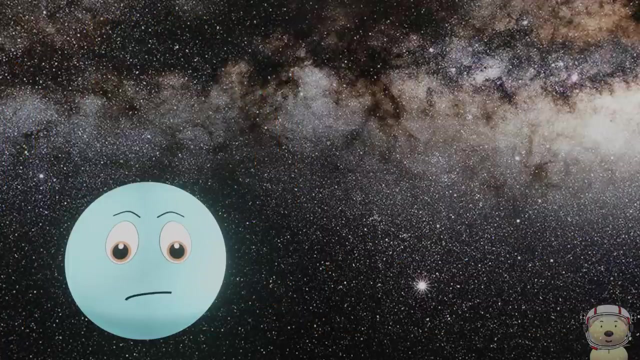 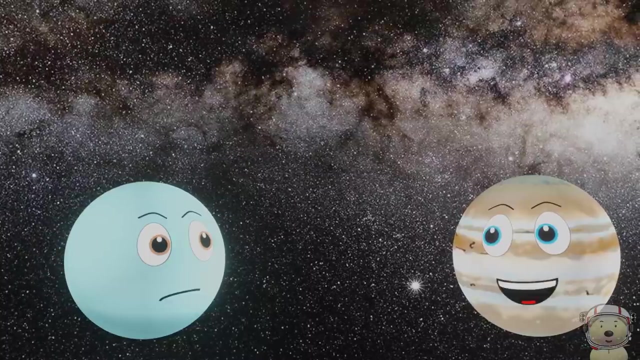 Hmmm, I could get used to this. No, No, No. Yes, Seventy years after discovering Georgium Sidus, it was decided to rename you to Planet Uranus. Oh no, What was planet Uranus named after? Planet Uranus was named after the Greek god of the sky. 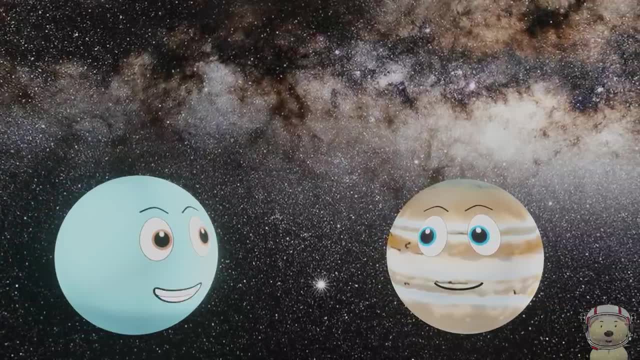 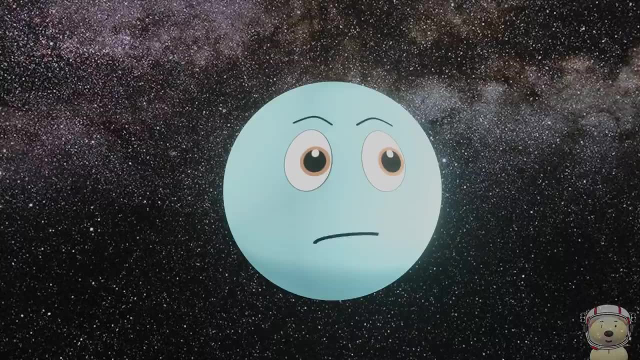 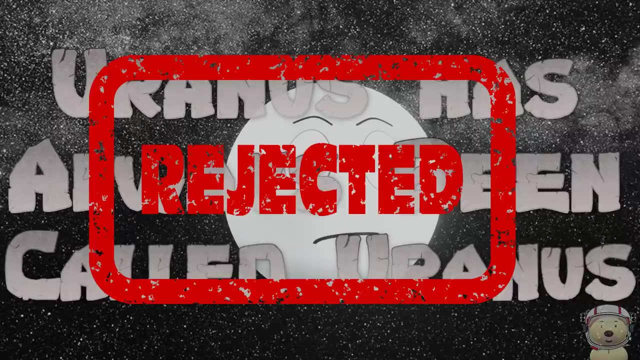 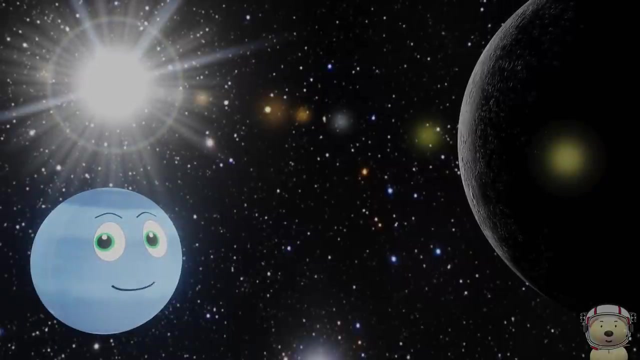 To be honest, I think I'd rather be called George or Humphrey, or What about Jupiter Junior? No Fact checked. Mercury is the hottest planet. Some people think that because Mercury is the closest planet to the sun, it must be. 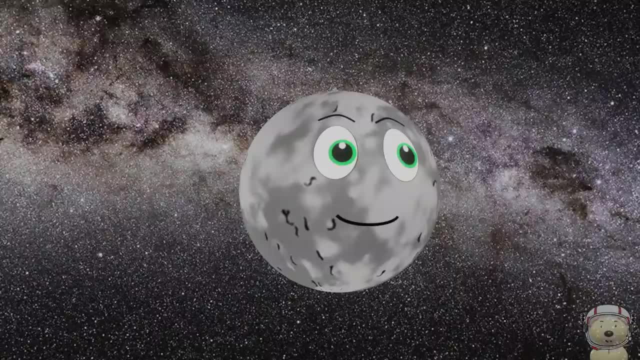 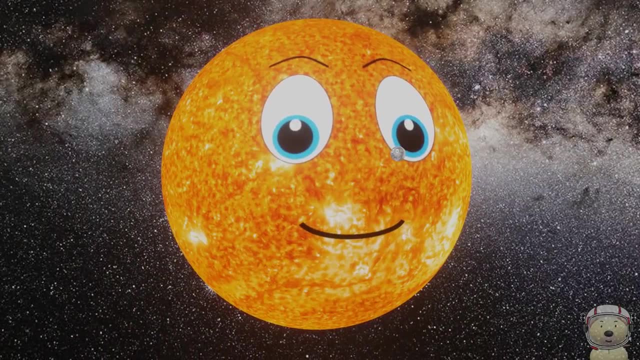 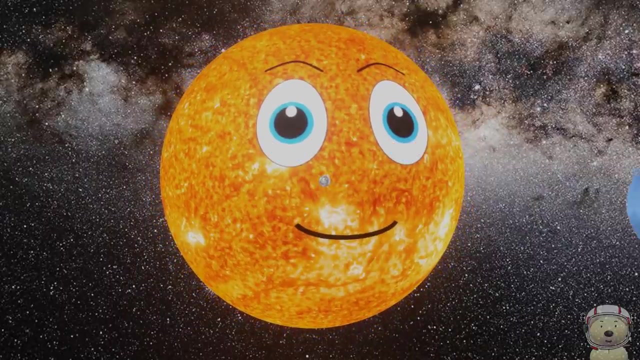 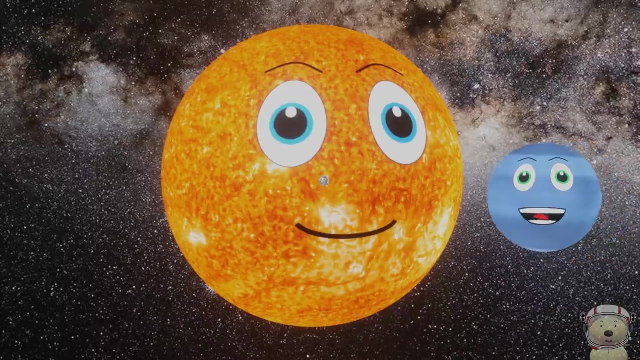 the hottest Wrong. It would make sense if Mercury was the hottest planet, as it is the closest, but that is just not true. What? But I'm boiling- look how close I am. I know Mercury, But in fact, Venus is the hottest planet in the solar system, even though it is about 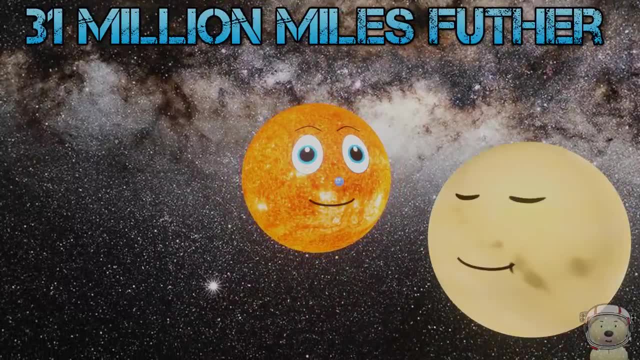 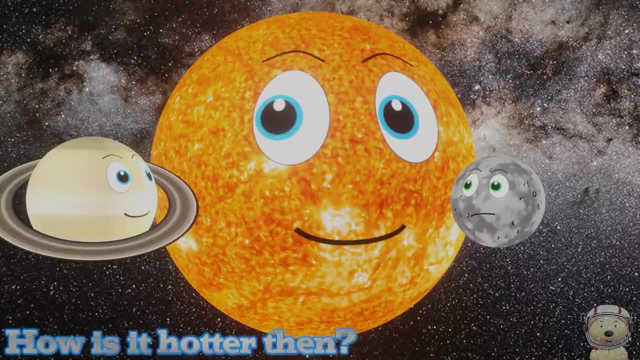 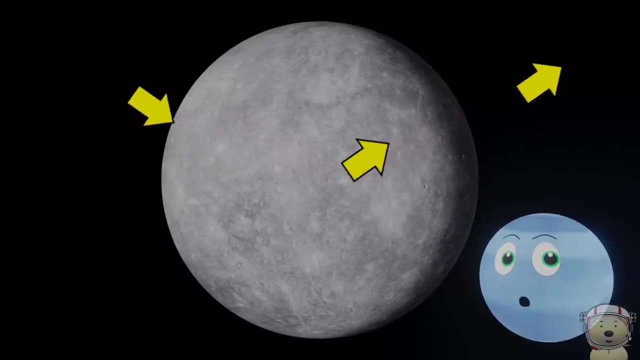 31 million miles further from the sun than Mercury is, Oh man, not fair. How is it hotter, then? Because it's so close to the sun, Mercury is the hottest planet in the solar system. Mercury has little atmosphere and no clouds around it, so the heat leaves the planet after.